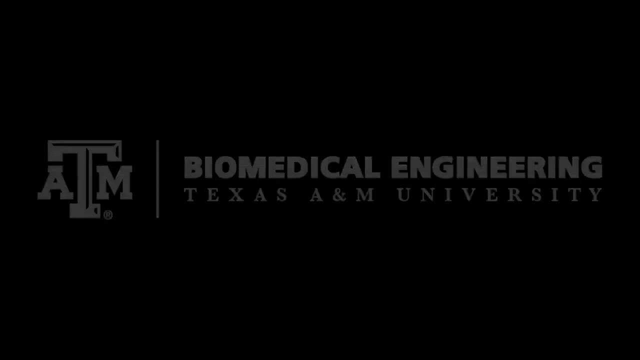 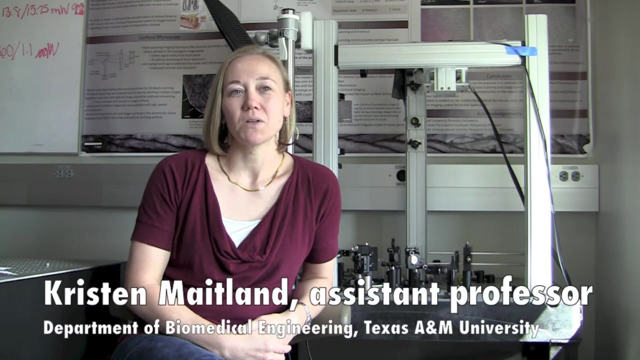 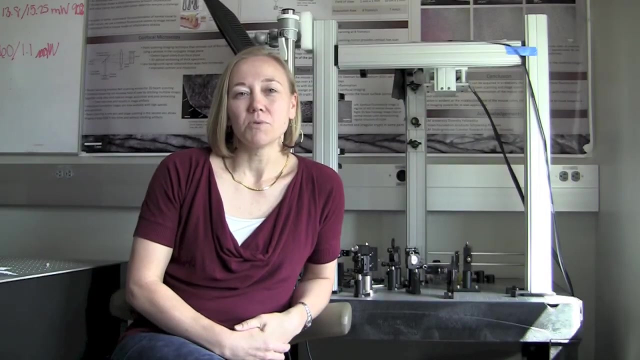 Hi, I'm Kristen Maitland. I'm an assistant professor in the Department of Biomedical Engineering at Texas A&M University. Currently, in my research lab, we're developing a new technology to improve early detection of oral cancer. Our approach is to combine two optical technologies. 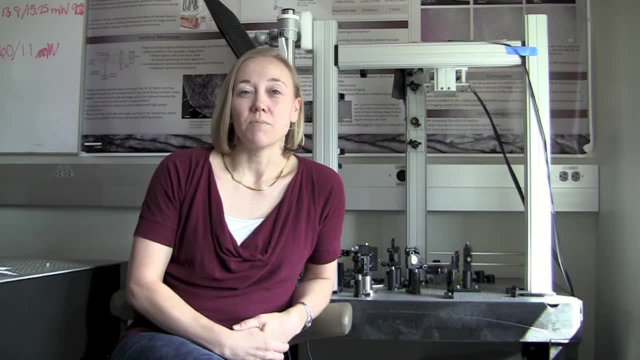 to provide information to the clinician, both on the macroscopic and the microscopic level, to improve the clinician's ability to provide an accurate diagnosis. When a dentist or a clinician examines a patient's mouth, they're basically using their eyes to sense or to 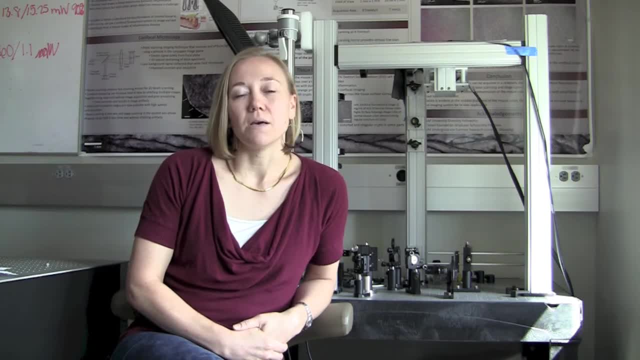 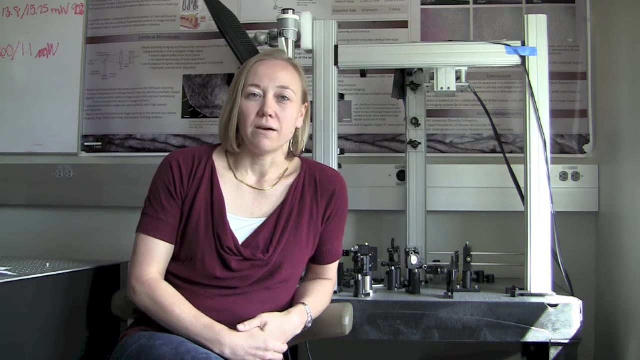 detect lesions within the mouth. The challenge with this is that patients frequently come in with lesions that surround the entire oral cavity or a large portion of the oral cavity, and these can be heterogeneous. where there might be precancer that could be hidden within a bed of. 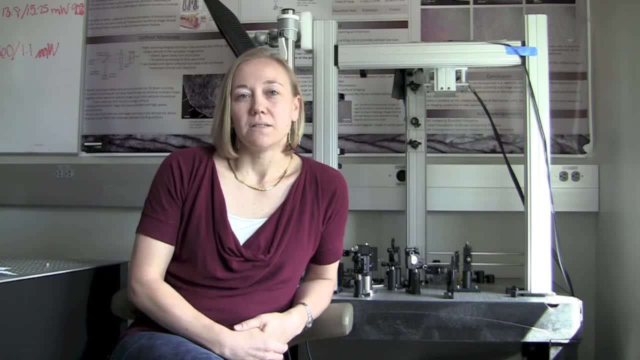 benign tissue. So what the doctor does is they look at this tissue and they try to decide what is the most severe case of abnormal tissue. They cut out that tissue using a biopsy tool and they provide that tissue to a pathologist. The pathologist slices the tissue and they 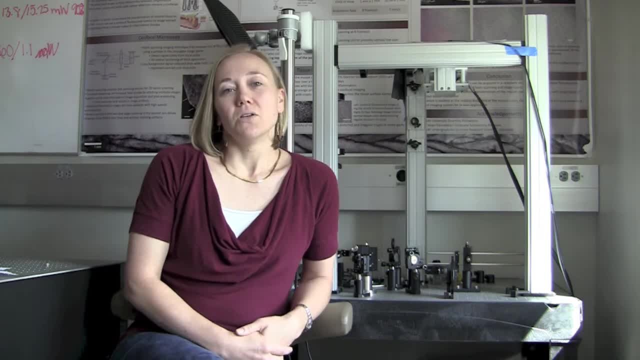 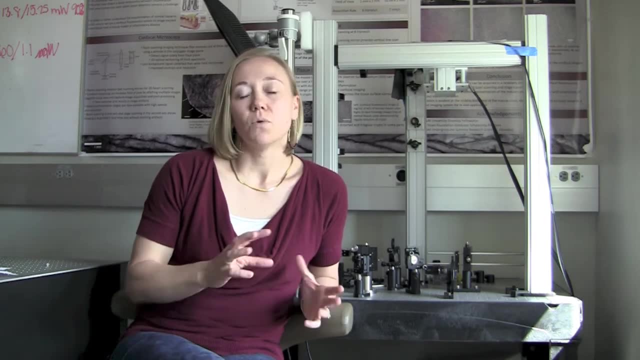 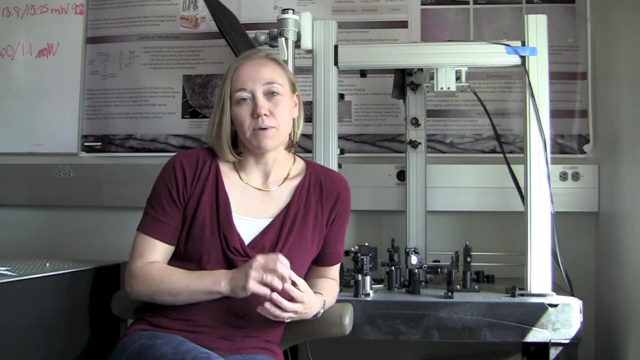 look at it in a microscope. First they look at it in a macroscopic scale where they're looking for overall tissue And they're looking for changes in the structure and in the biochemical composition. Then they zoom in using the microscope with a higher magnification objective lens and they're 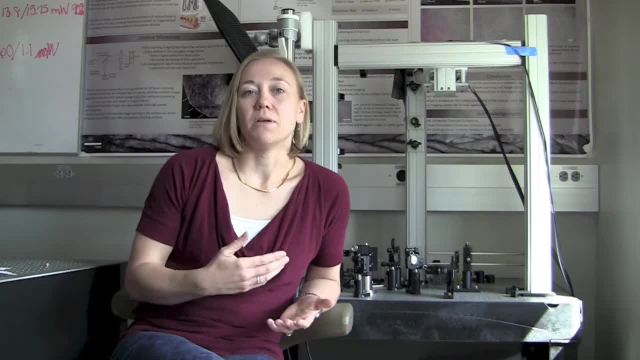 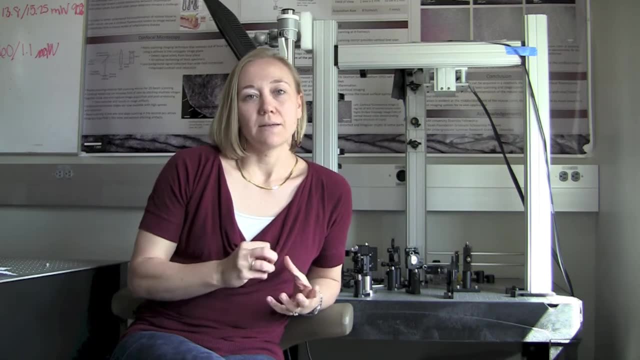 looking at the cellular features to look for changes that happen with precancer, that can indicate precancer. The challenge is, this small piece of tissue is meant to represent the worst state of disease within the whole oral cavity. So what our main idea is is that 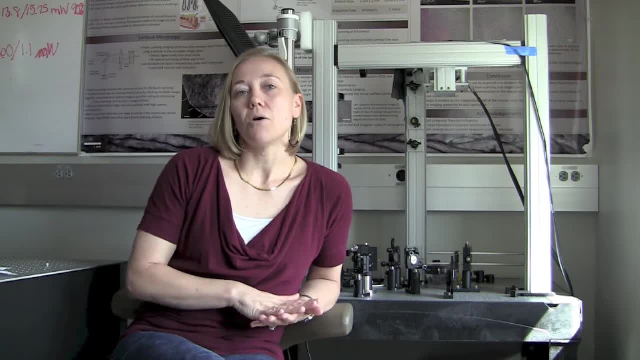 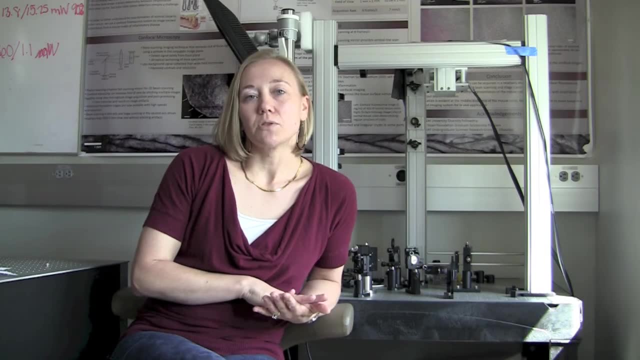 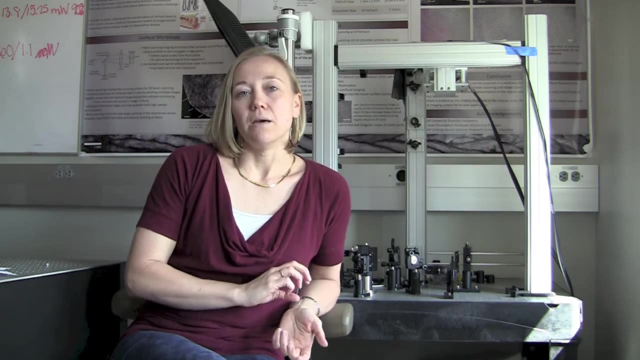 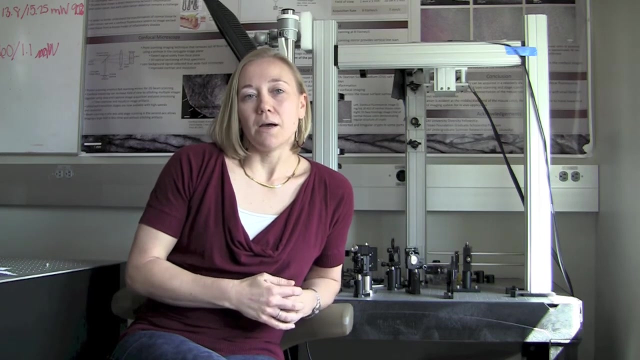 we want to provide more information to the clinician to help them select the most severe site within the oral cavity. To do this we are using two new optical technologies. One is called fluorescence lifetime imaging, which will provide some of the biochemical information. that provides metabolic information about the tissue on a macroscopic scale. And then 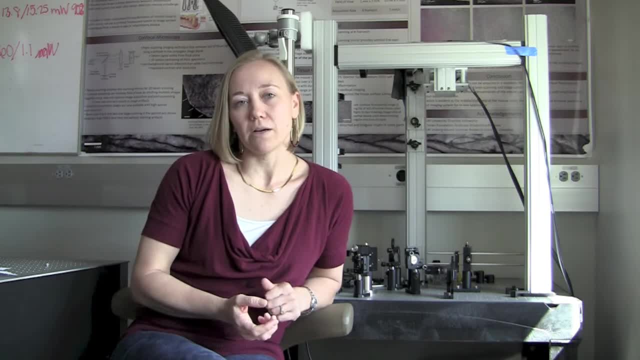 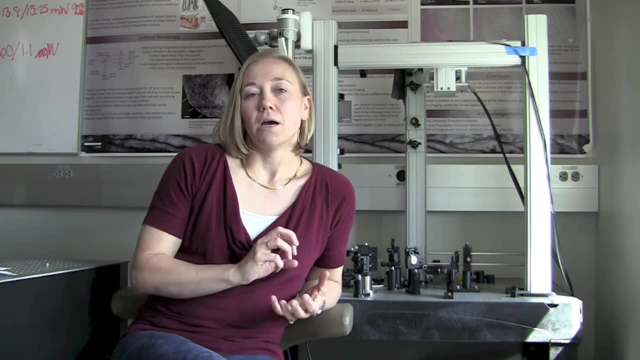 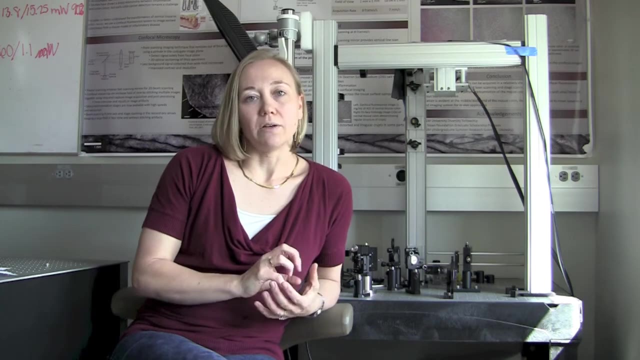 we use a technology called reflective imaging And it's going to help us identify the worst reflectance- confocal microscopy that provides high-resolution imaging of cellular structure. so we're looking for changes to the nuclei of the cells, where we're trying to identify if they're getting larger or more crowded, which is 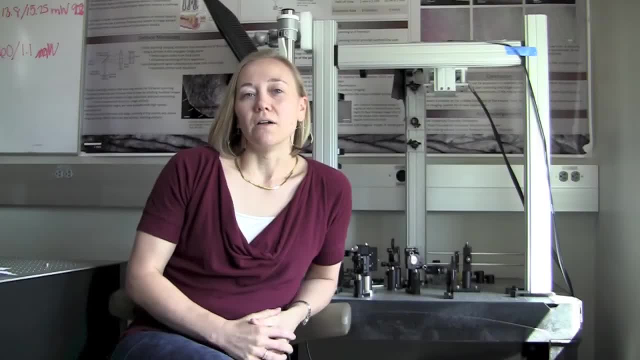 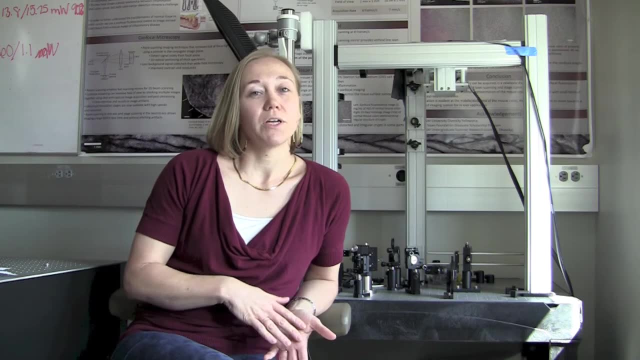 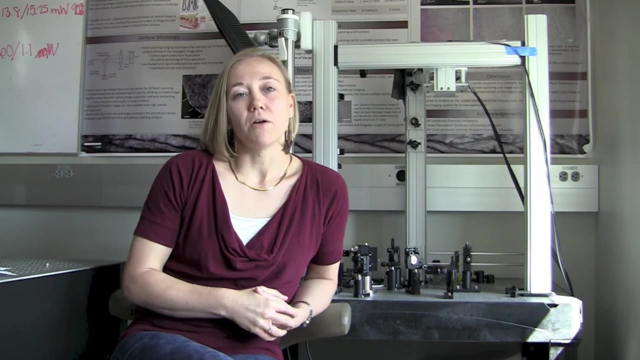 indicative of pre-cancer development. so overall, our imaging system is providing new information to the clinician. we're hoping that this can provide a more accurate and rapid diagnosis by providing real-time information to the doctor, and it may be applied to other applications such as monitoring. 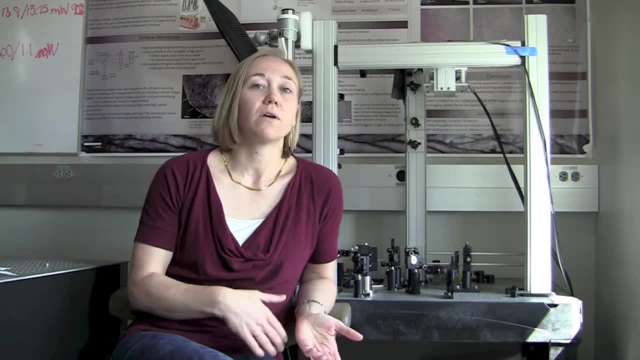 treatment. to provide real-time feedback to see whether a therapeutic agent is providing the desired effect on the cancer. 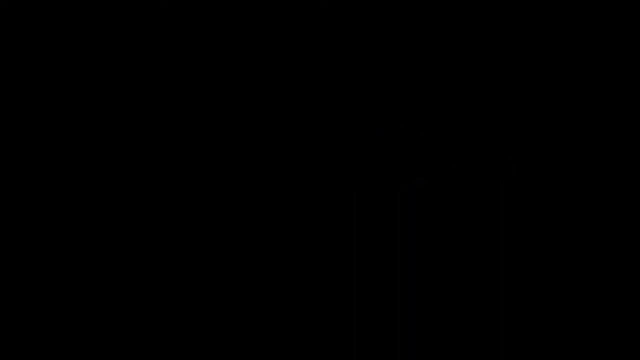 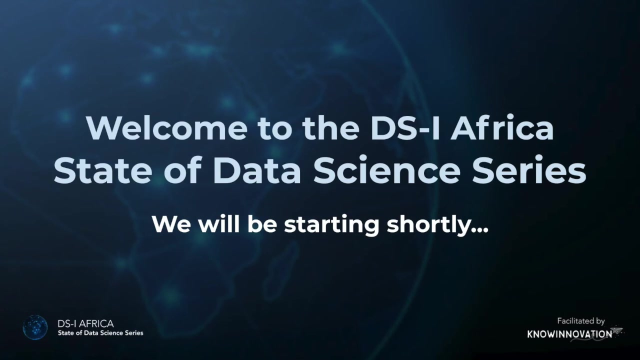 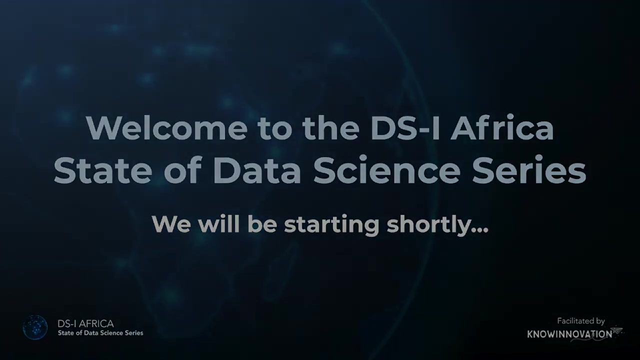 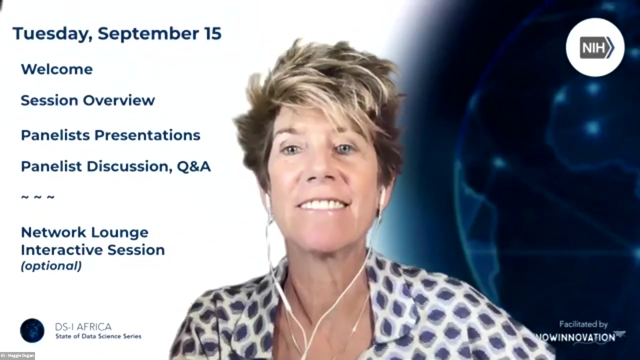 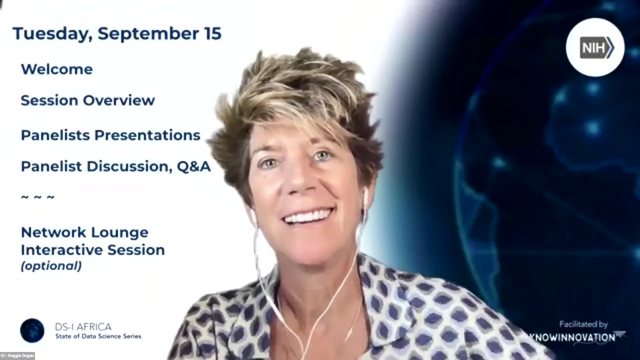 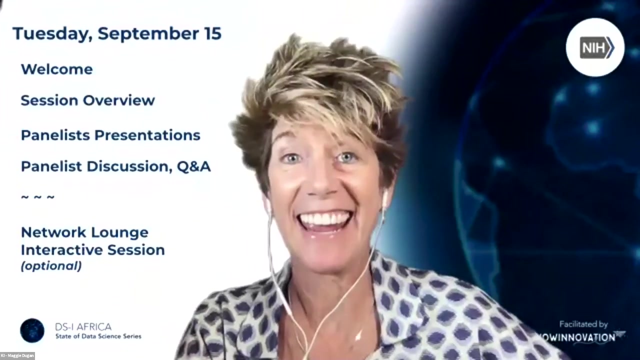 Good morning and good afternoon and welcome to the first webinar in a series of the State of Data Science in Africa. This is hosted by the National Institutes of Health Common Fund. My name is Maggie Dugan and I'm here with my colleagues from Know Innovation. We're also known as KI, that's the KI in Kai Storm. we used to. 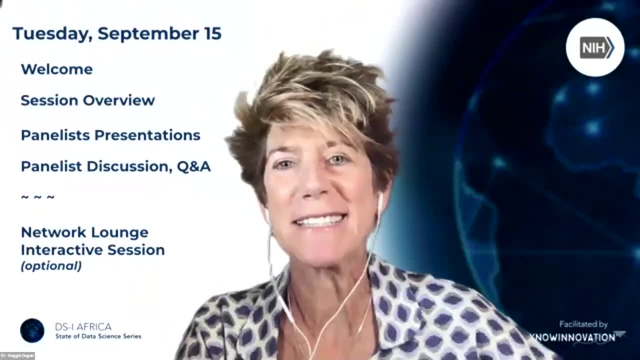 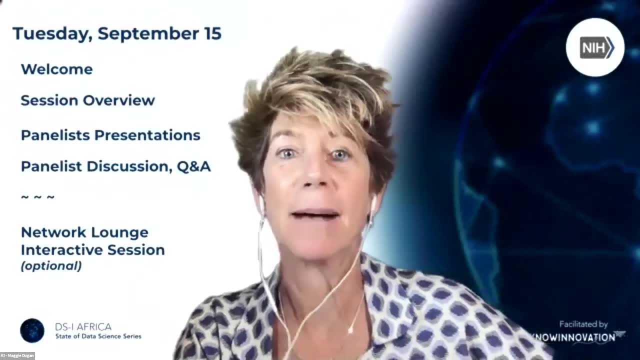 get here. We're a facilitation team that specializes in accelerating scientific innovation and we are very pleased to have been asked to help support this virtual event for the NIH Common Fund. Briefly, our agenda today: some welcoming remarks and tips for engaging successfully. 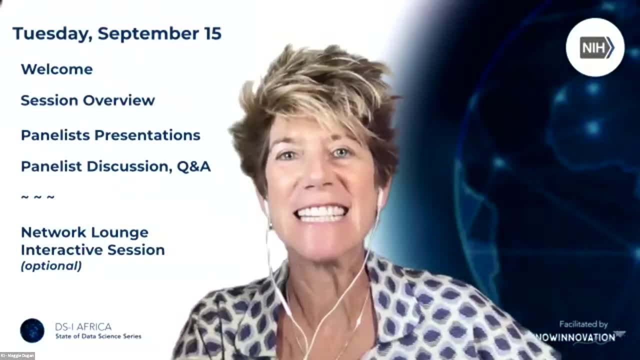 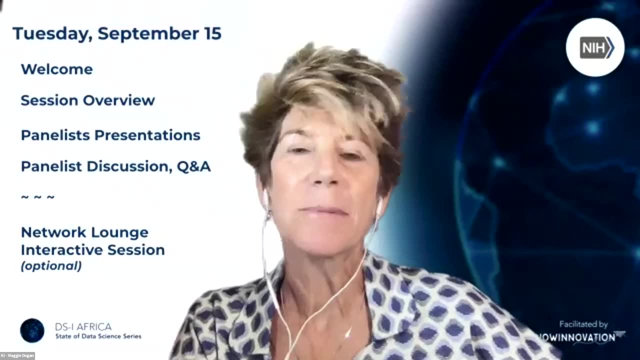 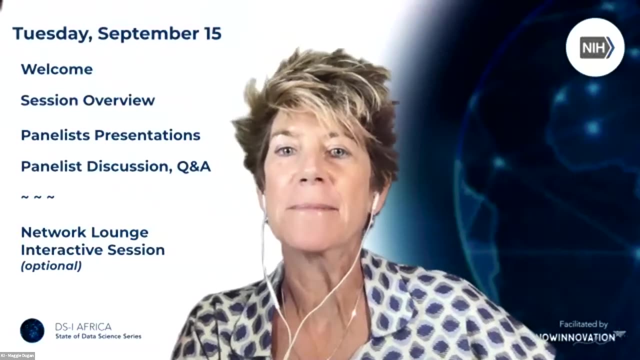 in the webinar, We'll have an overview of today's session on biomedical imaging acquisition and analysis from our moderator, Paul Perlman. This will be followed by 10 to 12 minute presentations from each one of our panelists. I'll let Dr Perlman introduce them and followed by questions.